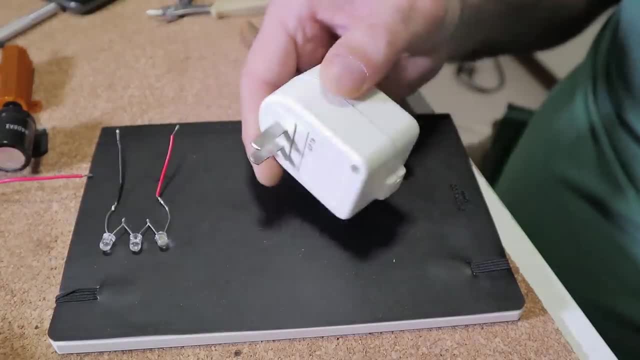 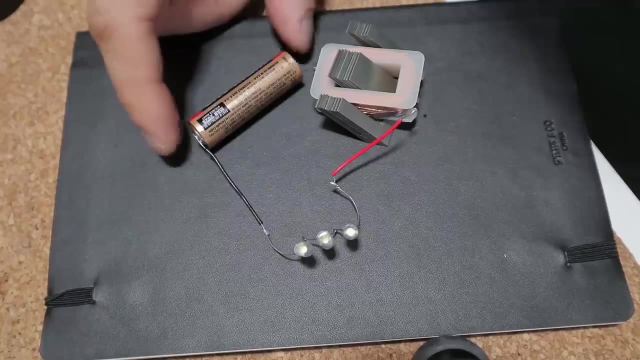 I have a regular transformer wall adapter not connected anywhere. You can use it as is or you can tear it apart and pull one coil of winding out. Either way is fine. Now the positive of the battery goes to the coil. that goes to the positive of the LEDs and returns to the battery. 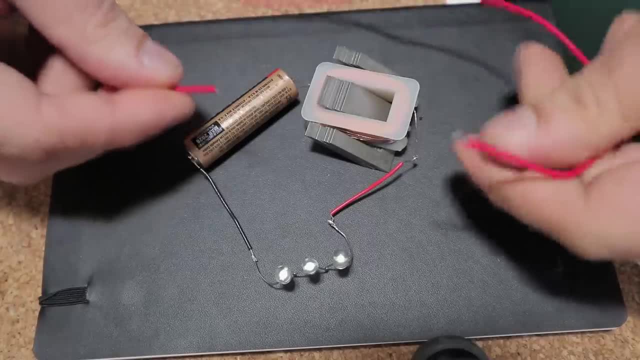 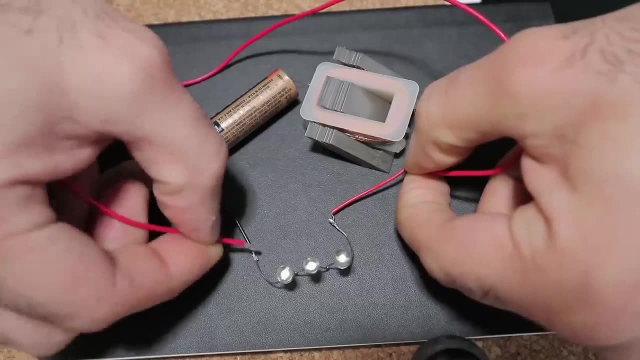 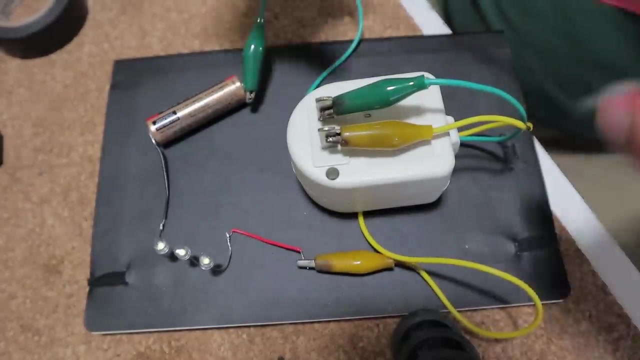 The battery still can't do sh**. but now, if I short across the LEDs with a piece of wire and let go BAM, I have nine volt pulses across them and they turn on. And here I can replace the coil with the wall adapter and doing the same thing, it's even brighter. 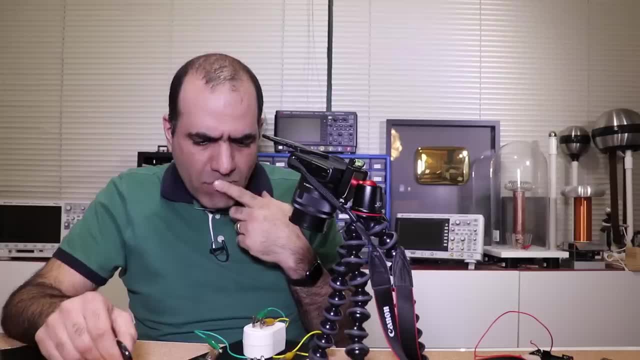 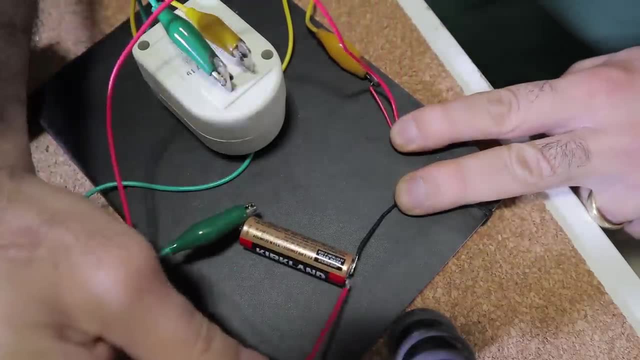 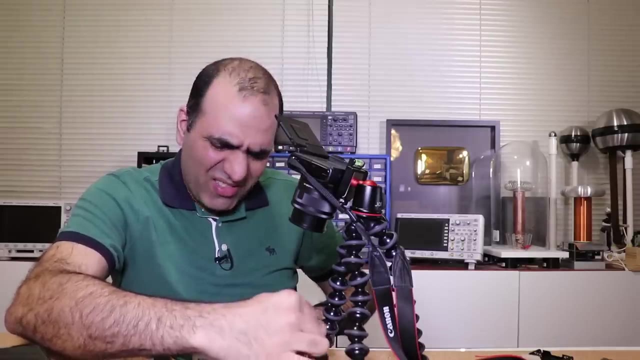 Doo-doo-doo-doo-doo Magic. I wonder if it can shock me Here. instead of the LEDs, I put my fingers across the wires and short across my fingers. Eh, Ow, Yeah, I mean, I can feel it. so there are pulses of high voltage. 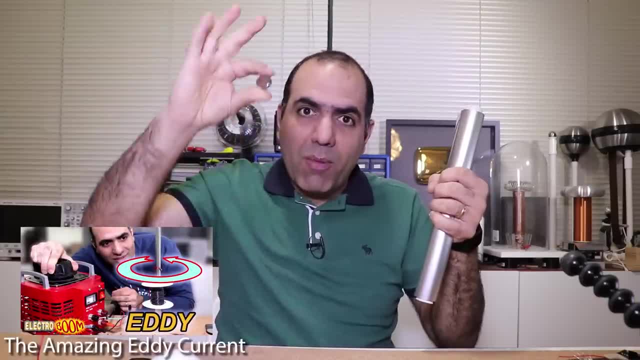 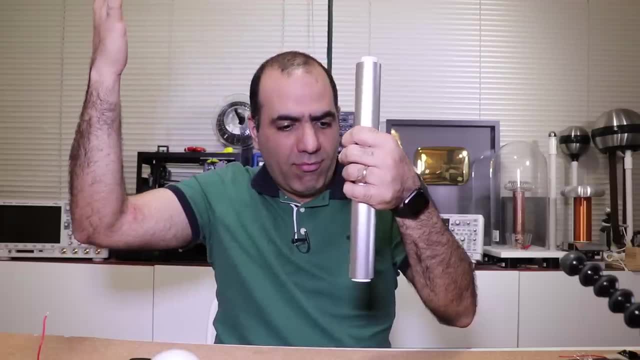 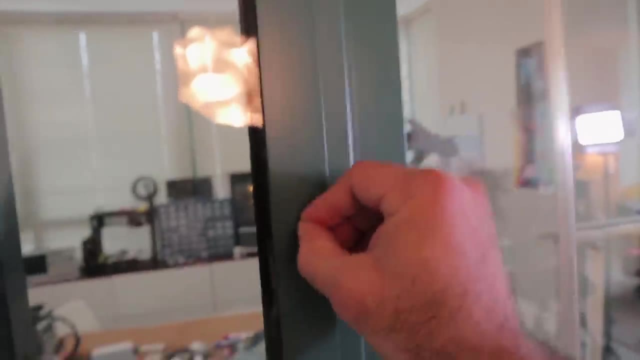 There's a new way to get shocked. I've shown you before that neomedium magnets drop like a rock in air, But if you drop them through a roll of aluminum foil they drop very slowly But similarly look. this frame is also made of aluminum and my magnet has north and south on the surfaces. 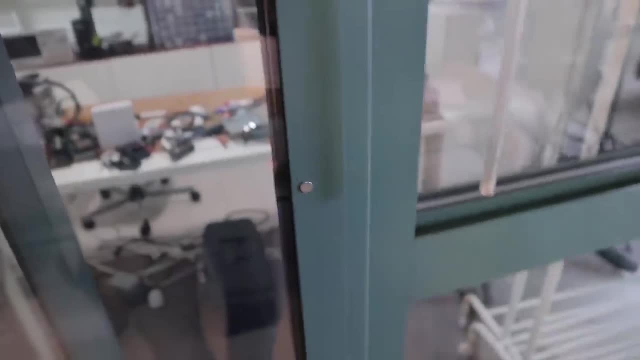 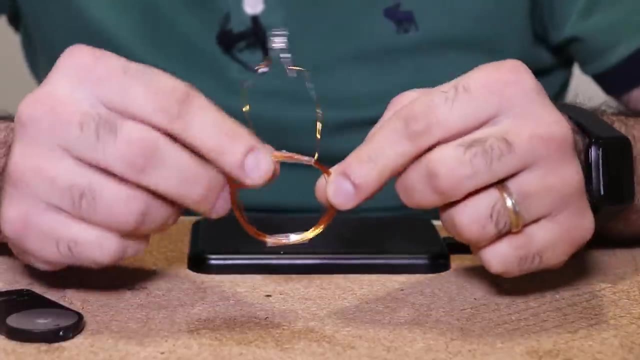 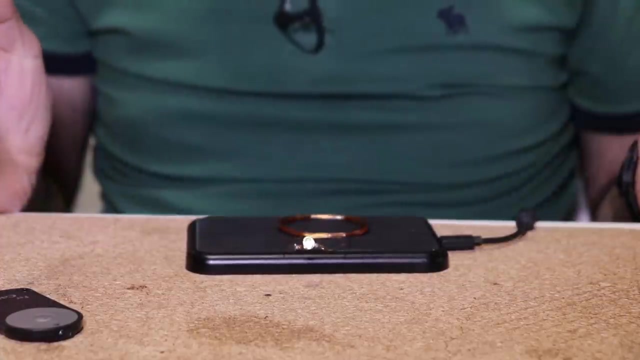 And if I put it on and let go See, It goes down slowly. Doo-doo-doo-doo-doo-doo Magic. You can make a few turns of winding and connect an LED to its end and drop it on a wireless charger and BAM. 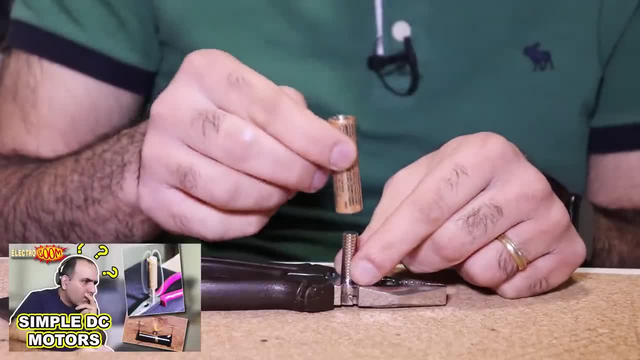 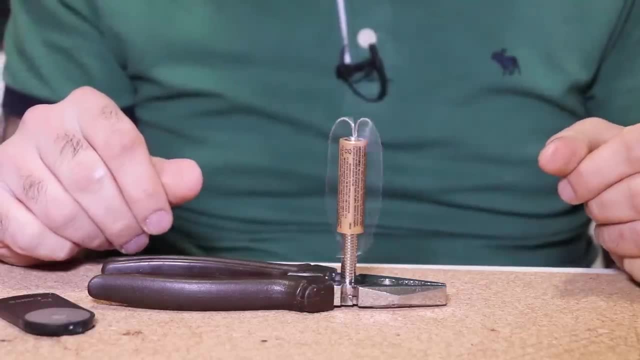 Doo-doo-doo-doo-doo Magic. You stick a battery on a magnet and short the battery using a piece of wire like this, and it starts turning Doo-doo-doo-doo-doo-doo Magic. 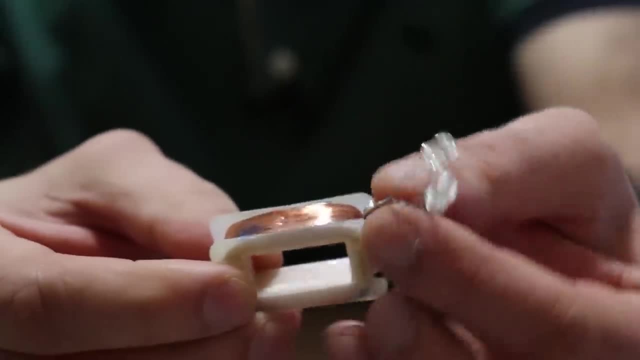 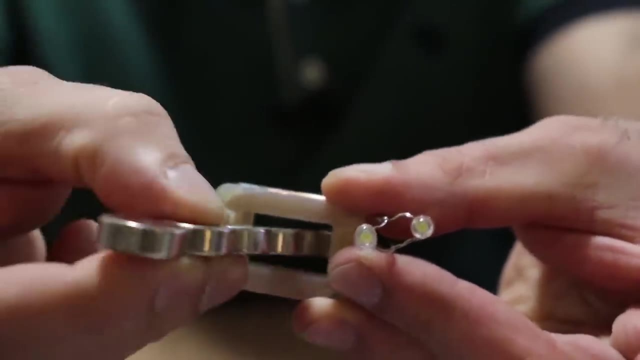 You connect two parallel reverse LEDs across a coil and pass a magnet through it. Doo-doo-doo-doo-doo-doo Magic: You connect two parallel reverse LEDs across a coil and pass a magnet through it And ping-pong, ping-pong, ping-pong, ping-pong. 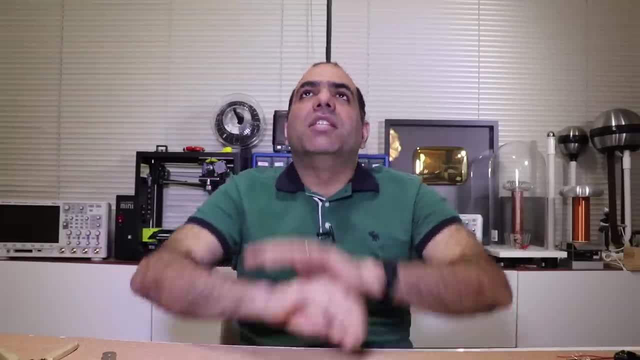 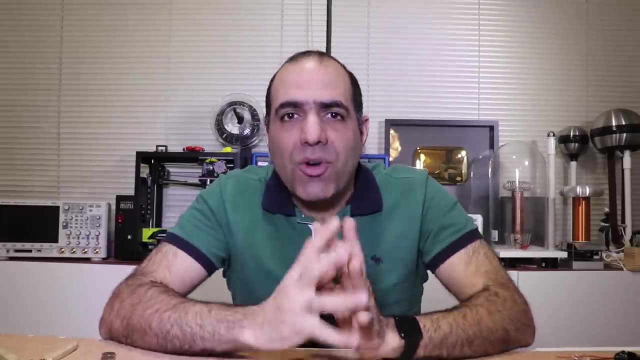 Magic, Of course I joke. it's not magic, It's magic. Oh, it's magnetism. Stay with me to the end to understand what's going on. Stay. Magnetism is quite simple, at noob level, which we strive for here. 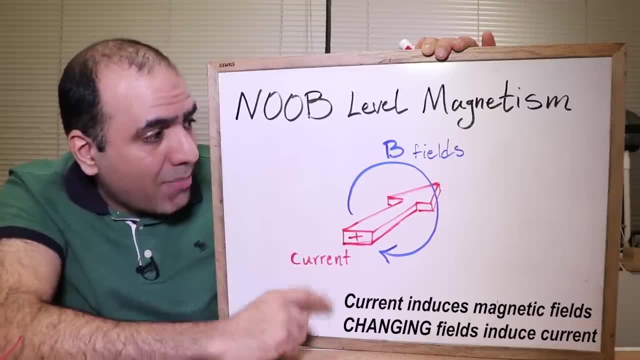 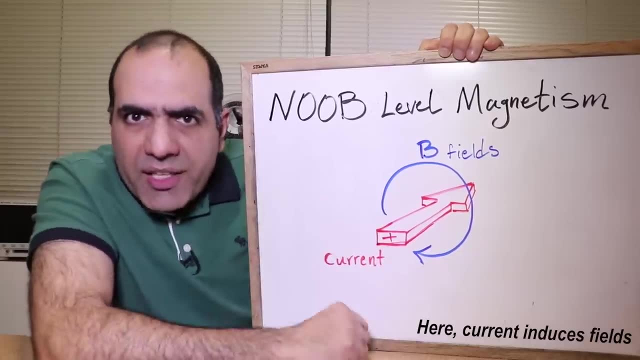 When you have charges moving in a direction, you have current and magnetic fields wrap themselves around that path, like this, going to infinity. This follows one of the right-hand rules, where the thumb shows the direction of current, which is the flow of positive charges, or reverse of electron flow. 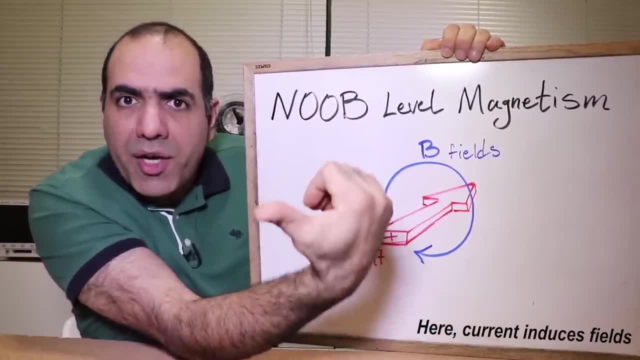 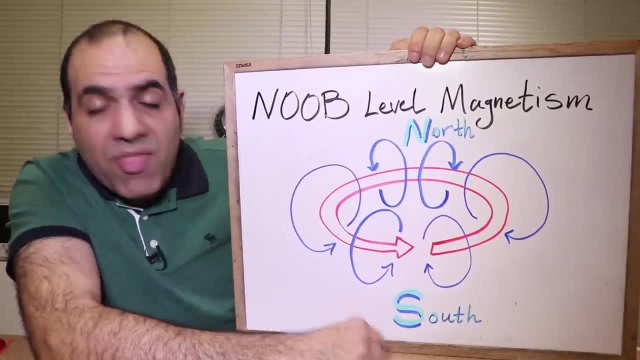 And other fingers show the direction of fields wrapping around the wire. So if the current runs in a loop like this, magnetic fields wrap themselves all around the wire like this, And that's why some metals like iron have stronger magnetic properties and are called ferromagnetic. 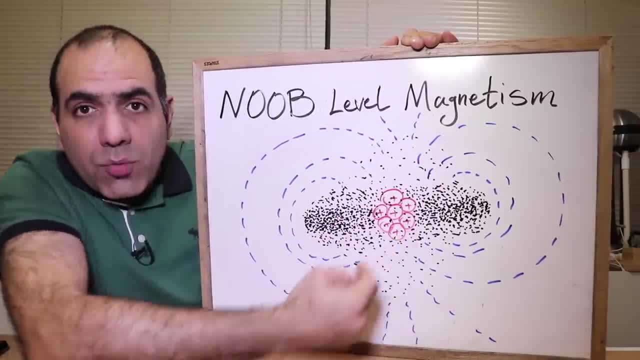 It's because this cloud of electron turns around the wire like this. It's because this cloud of electron turns around the wire like this. It's because this cloud of electron turns around the wire like this. It's because this cloud of electron turns around the atom core in a more defined direction and turns the atom into a tiny magnet. 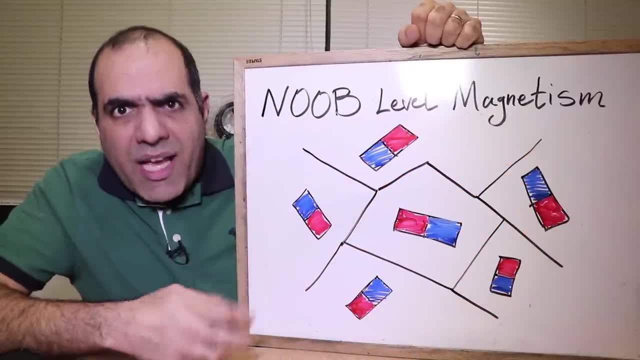 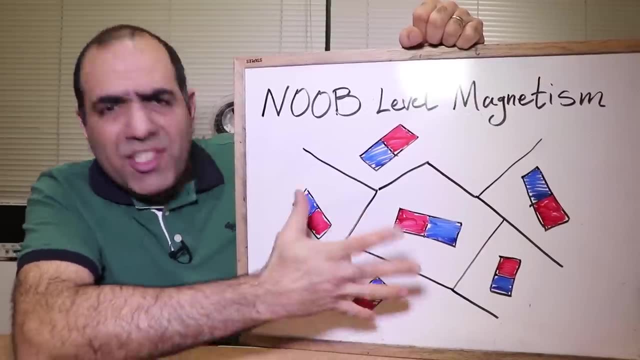 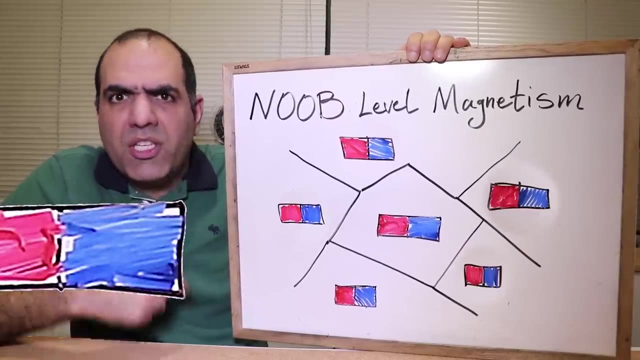 But see when the molten iron cools down, it solidifies and crystallizes into this patchy crystal form, with every tiny patch having a random magnetic direction. So all these random directions cancel each other and the iron is neutral. If you bring a strong magnetic field close, you force these to rotate and align with the field. 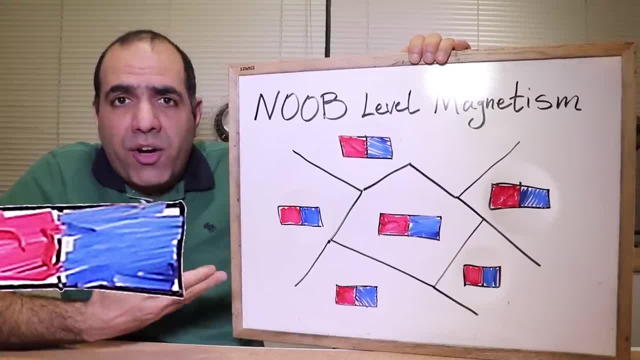 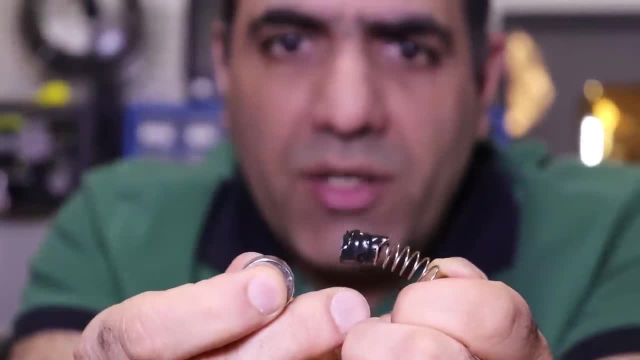 which not only magnifies the original field, it turns the iron into a magnet. But it's like these tiny magnets are stuck on a spring And if you bring an external field close they try to align themselves. And the stronger the field, the further they align until they fully align. 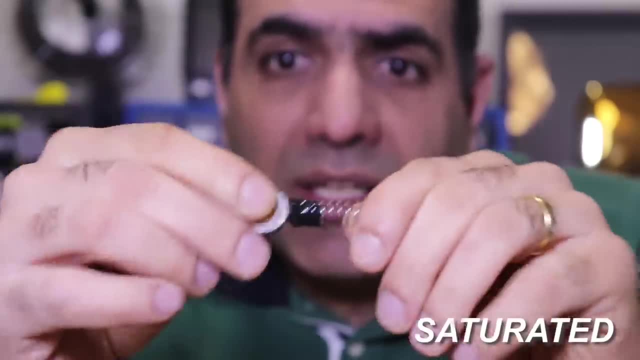 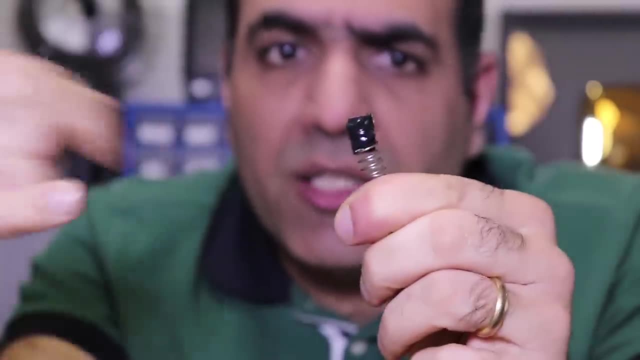 This is when the magnetic material is saturated, meaning that stronger external field won't make any difference in their magnetism. And when we try to remove the external field, they try to spring back, Unless too much force has bent them permanently out of shape. 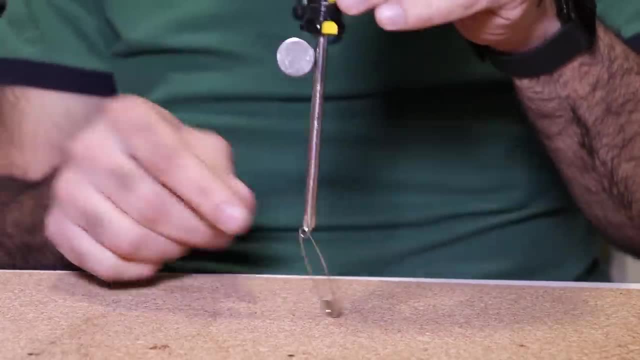 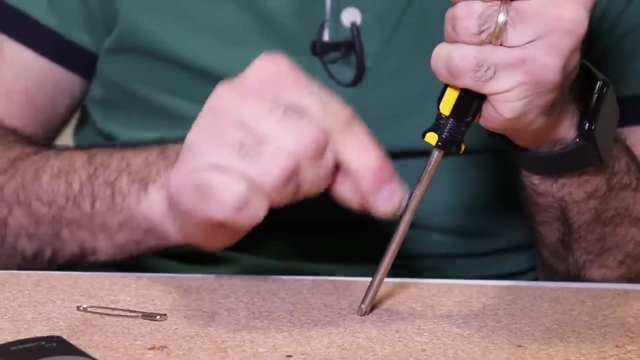 Unless too much force has bent them permanently out of shape. Unless too much force has bent them permanently out of shape of ferromagnetic material and you connect a magnet to it, it becomes a magnet too, and if your source field is strong enough, you can bend those tiny springs out of shape and make a more permanent. 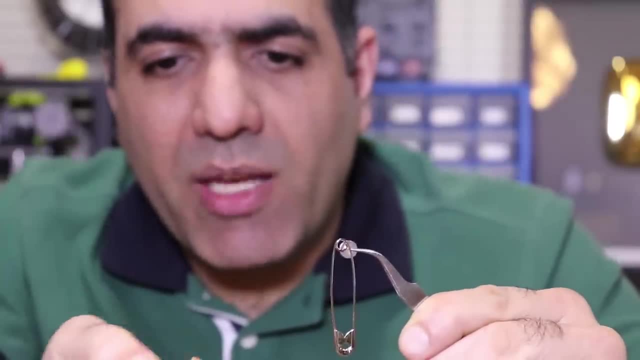 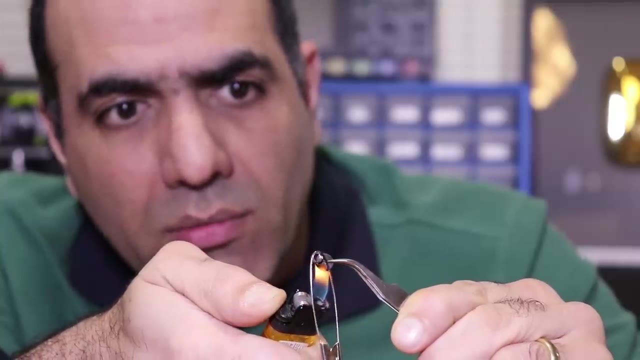 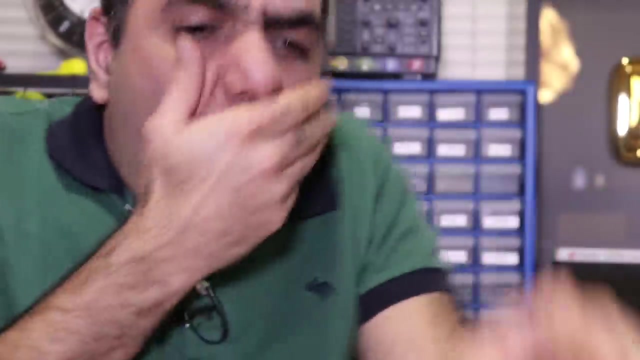 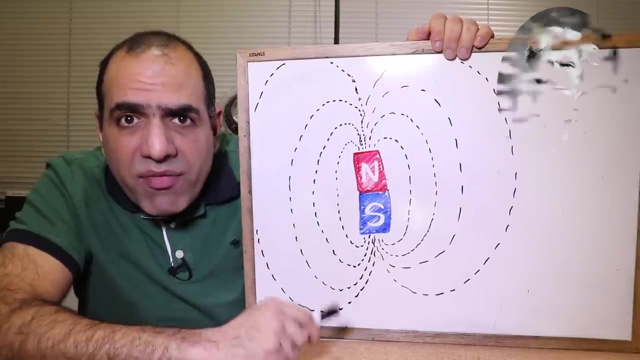 magnet. of course, heat is the enemy of permanent magnets, because the structure shakes out of alignment and the magnet dies forever there. so don't overheat your magnets. goodbye love. not everything hot is kissable. it was michael faraday who was first able to imagine and observe magnetic fields as these. 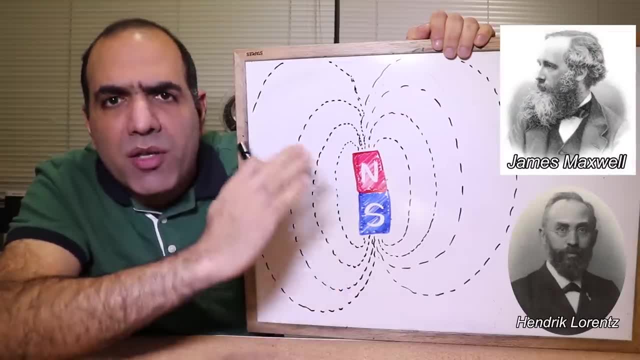 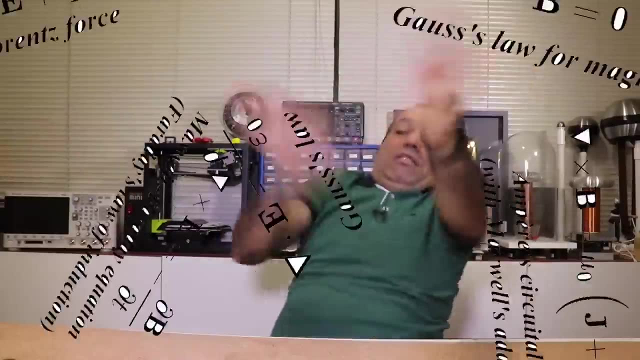 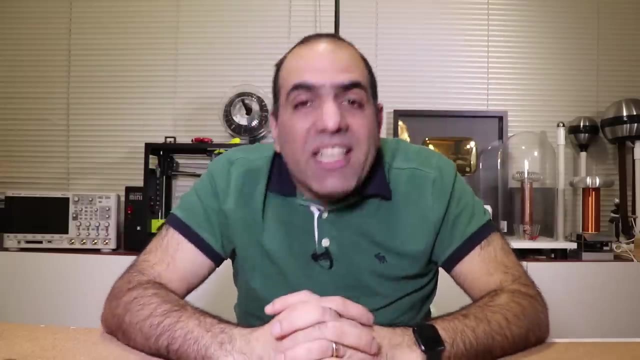 invisible lines. and then later, with the help of maxwell and some other scientists, they put together these complex equations to describe electromagnetism. forget about this. i'm supposed to be educated to be able to use these equations, but just seeing them hurts my brain. learn them at. 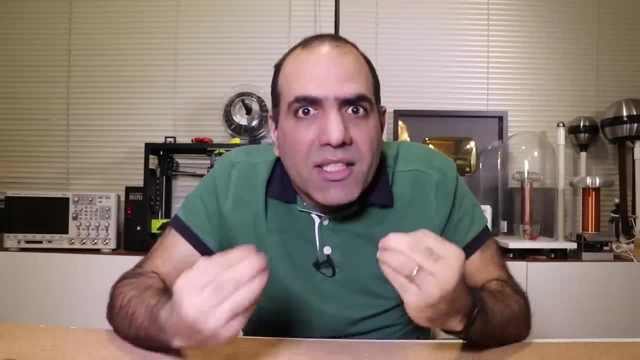 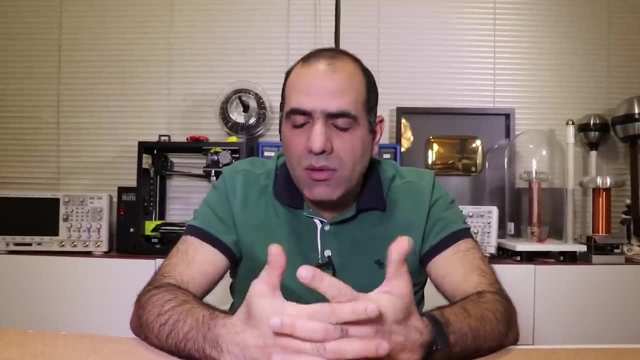 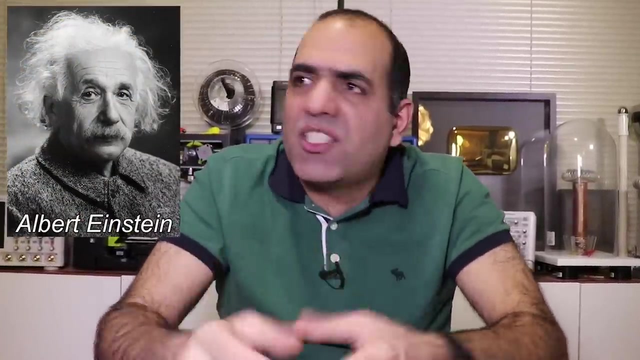 your own risk. but here i am, like you, to really feel magnetism in your heart. observing magnetism is quite simple, like my examples at the beginning, except that magnetism is fake. it's like the shadow of electric fields and it has something to do with einstein's theory of relativity. don't worry, i'm not going. 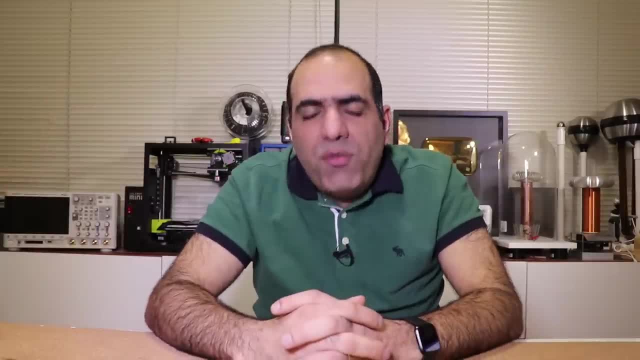 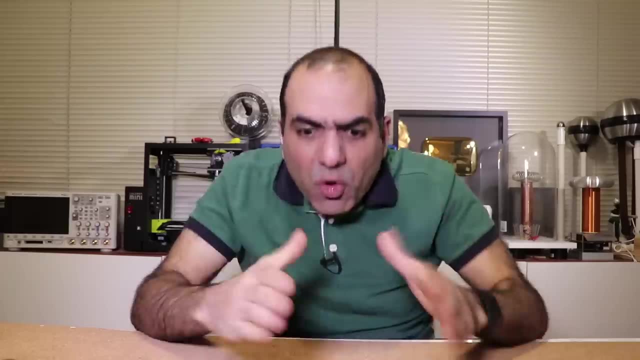 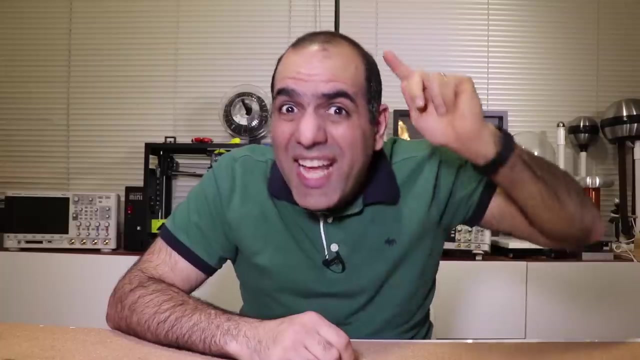 there, especially since i don't know what the hell is going on. if you're a professor with clarity on the subject, please help me and put me out of my misery. but for now, forget about everything complex and let's stick to primitive ways, knowing that the concept of magnetism is correct and makes our calculations. 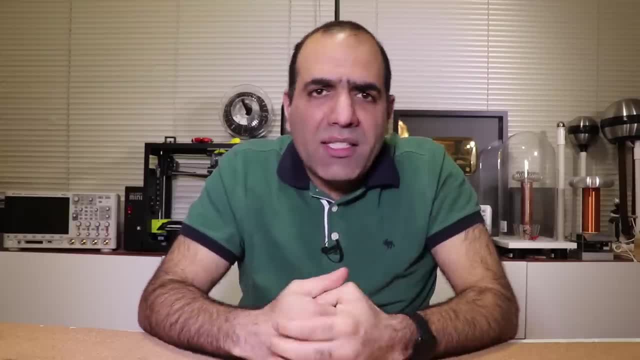 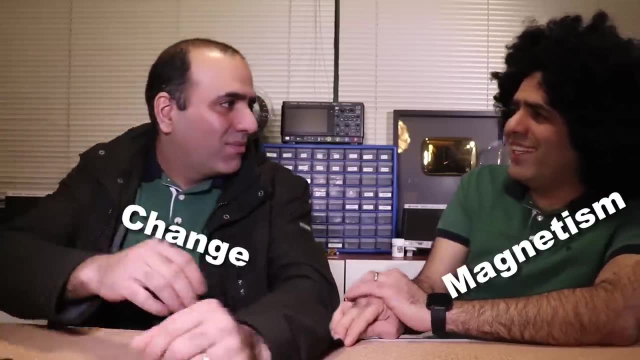 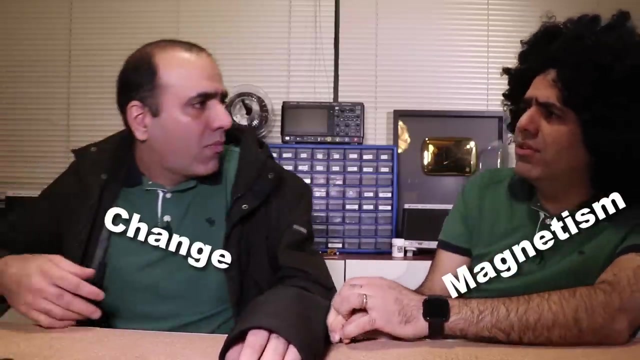 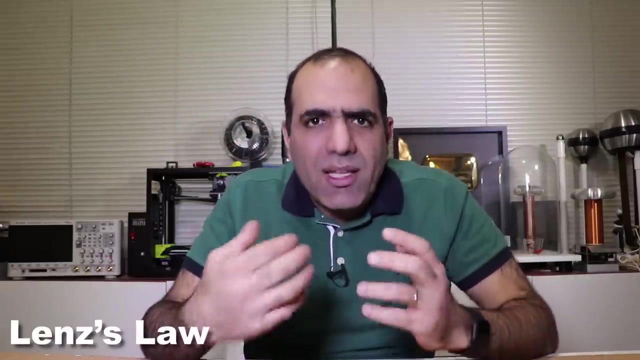 very efficient and simplified. so magnetism is like an annoying partner. it resists any change, like: let me just no, don't leave. okay, then give me a kiss. what the hell are you doing, your animal? the hell. let me just go, don't leave. for what the clip is trying to say is that in magnetism, according to lens law, anything that's 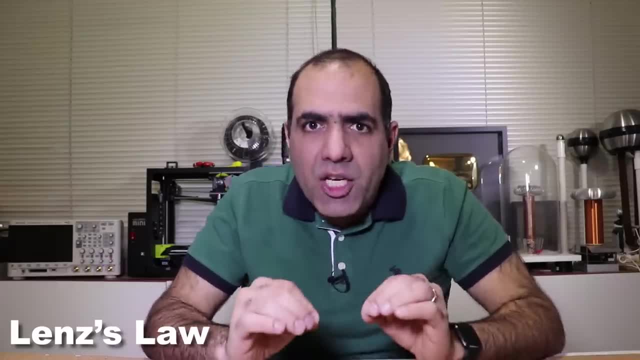 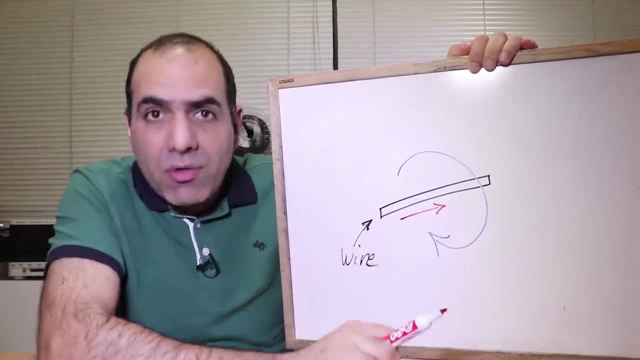 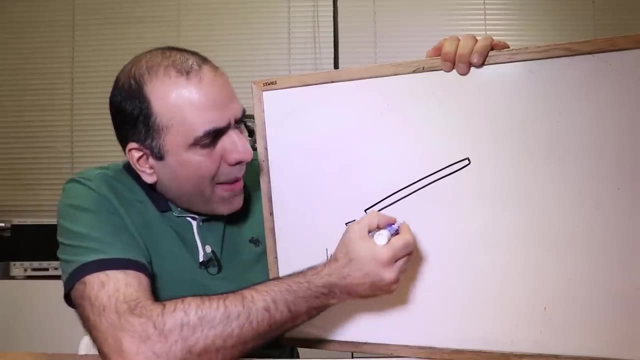 created due to magnetism opposes any changes in its creator. you raise current through a wire. it induces changing magnetic fields around the wire that create opposing currents in the wire. to reduce the changes in the source current, you change the magnetic fields around the wire and they induce a changing current in the wire. that creates a magnetic field around the wire that. 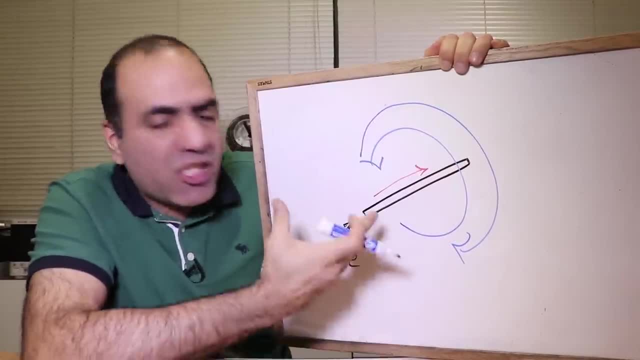 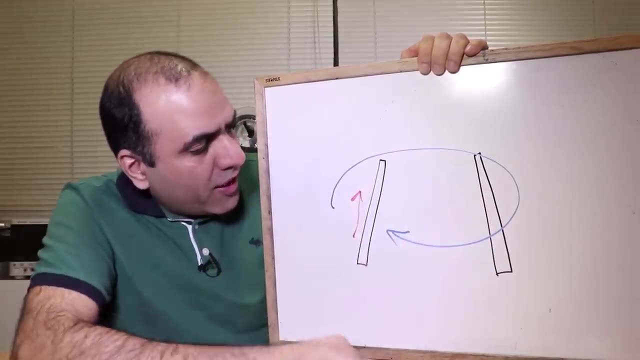 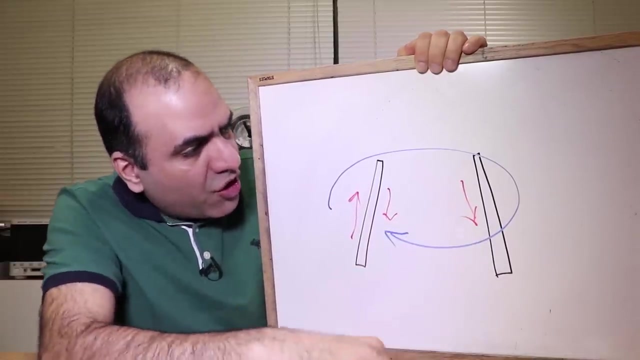 creates opposing magnetic fields. to stop the changes in the source field, you raise current through a wire. they create changing magnetic fields around it that oppose the source current. those fields wrap around another wire and induce a changing current that create opposing magnetic fields and reducing them so that they can't effectively oppose the 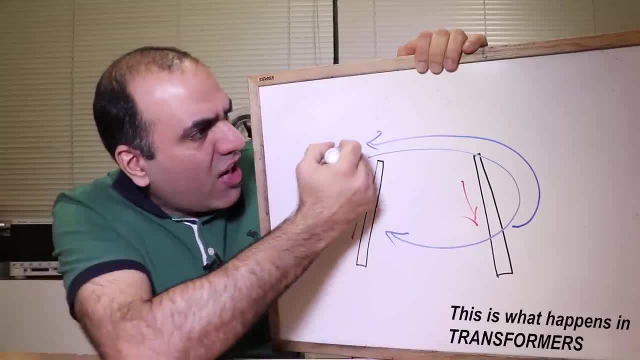 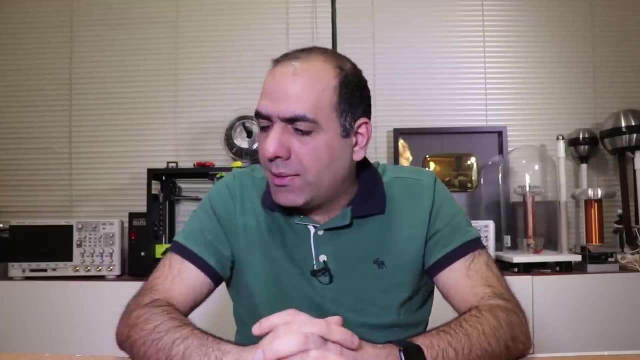 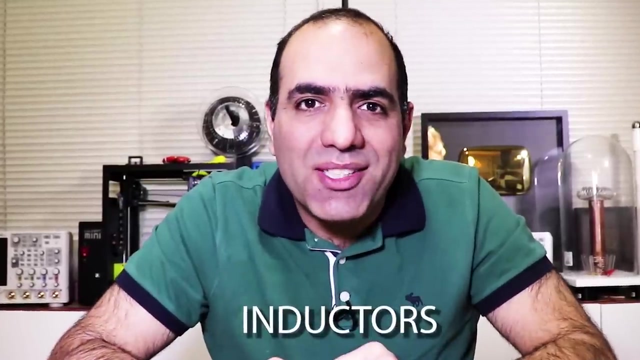 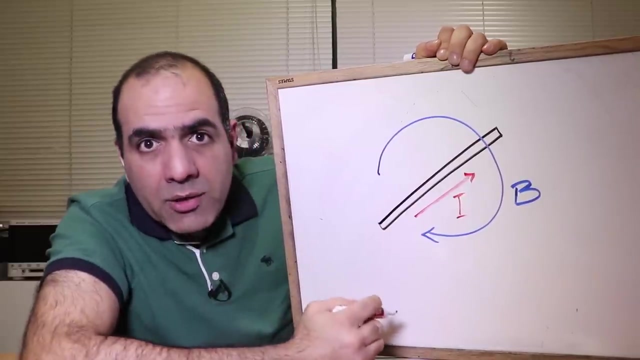 source current. so the source current rises again, creating even stronger magnetic fields so that It can maintain the output current. It's an opposition mess, But this feature of magnetic fields is what we use to create inductors and transformers. See, inductance is based on this property that the induced magnetic fields oppose the changing current by 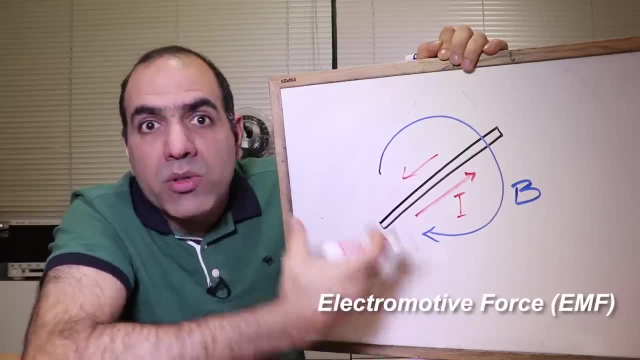 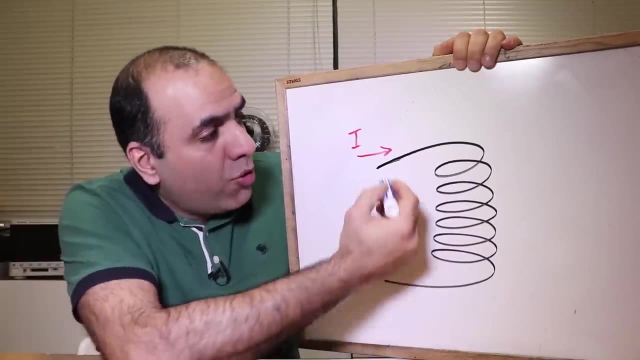 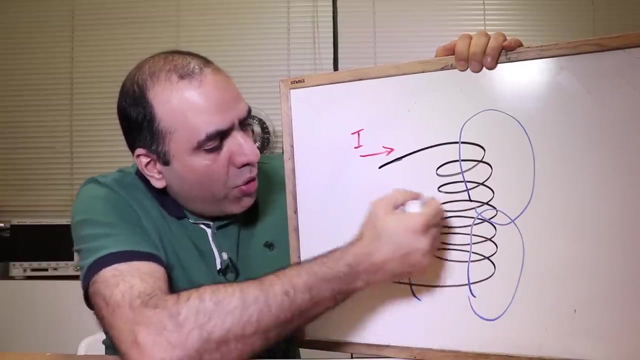 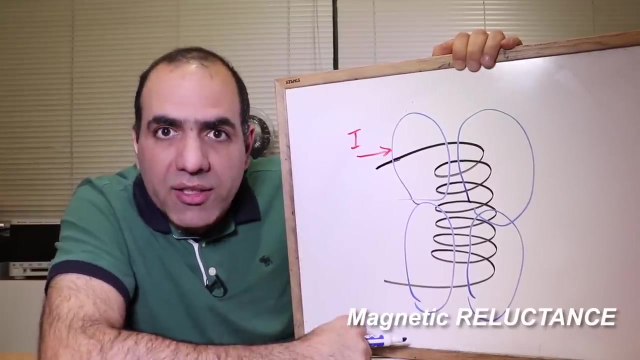 inducing an opposing force called Electromotive force. so every piece of wire has some inductance associated to it. But to increase this effect we loop a longer piece of wire like this, so that the fields created from each wire wrap around more wires, And this increases the inductance and so the magnetic reluctance against the change of current. 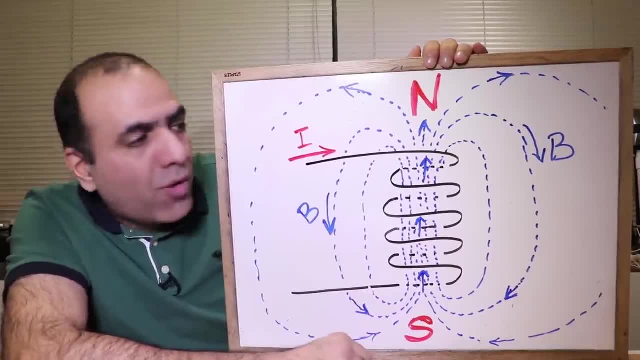 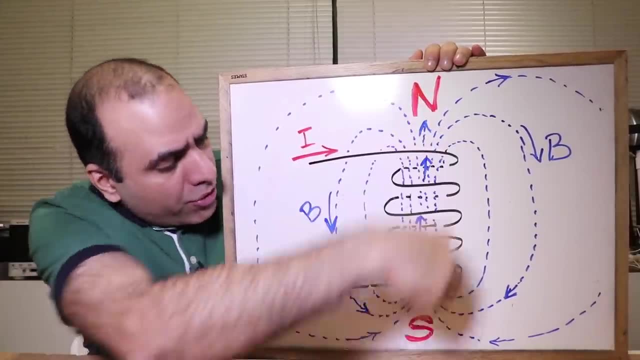 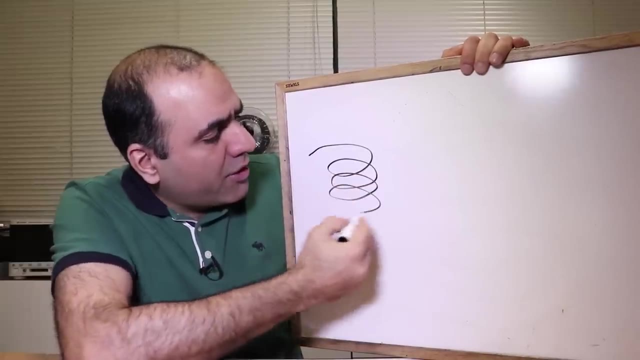 the overall magnetic fields around such an inductor, Which is also an electromagnet, looks like this, with the direction of the fields following the right hand rule and from north to south on the outside of the electromagnet And south to north inside, so increasing the number of turns. Increases the magnetic fields and raises the inductance. also, a larger radius increases the length of wire and so the inductance. and adding a ferromagnetic core like iron magnifies the magnetic fields and significantly raises the inductance. inductance is shown with capital L with unit of Henry named after Henry. 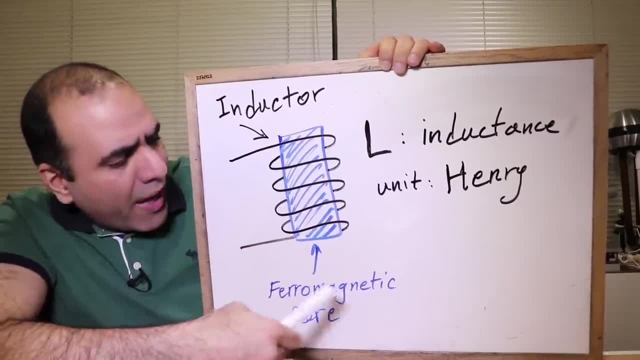 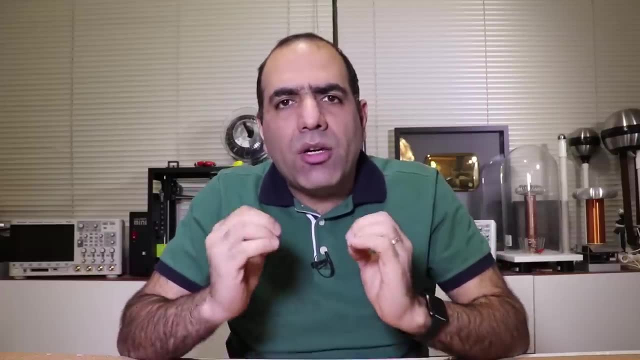 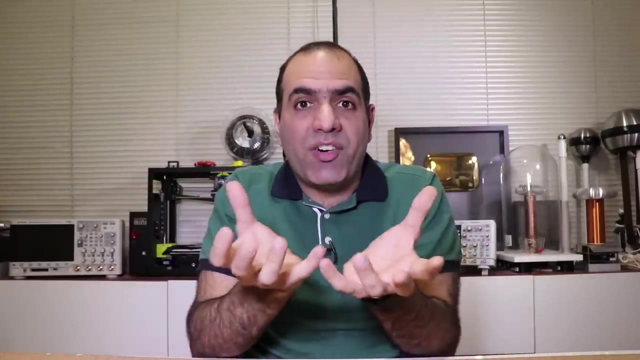 We can calculate inductance based on the coil geometry and core property, Which I don't care about. you can use online calculators. So, after all this description, what is an inductor good for? What an inductor does is that it stores energy in the form of magnetic fields in the space around it. Like I said, those fields oppose the changes in the source current, so they have energy to do it. It is like an elastic hose: if I push water current into it, It expands and a steady flow of current Goes out of the other side. but if I suddenly shut down the input current, the hose collapses and keeps pushing current out of the other side. 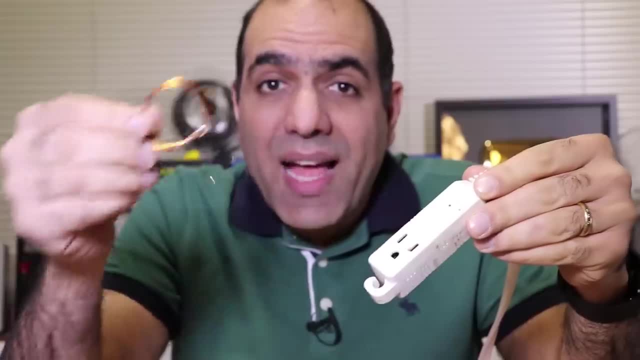 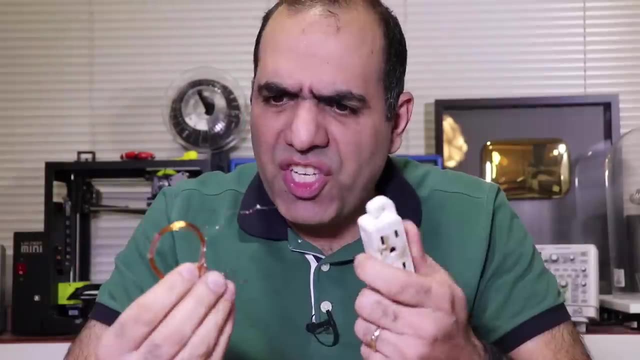 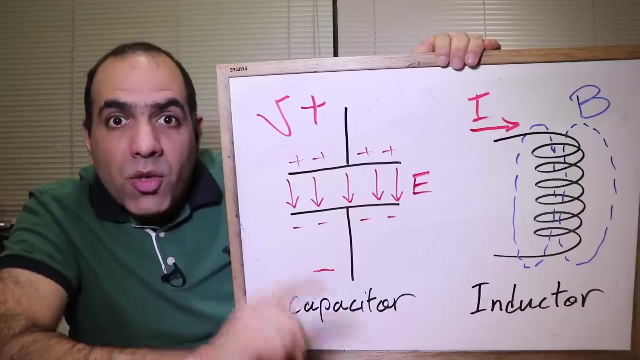 So it opposes the sudden change of current at the input and that's why they say a capacitor blocks DC But an inductor blocks AC, Which is inaccurate as hell. what's accurate is capacitor blocks DC but inductor shorts DC. So this is important in my previous Electro boom 101 episode. 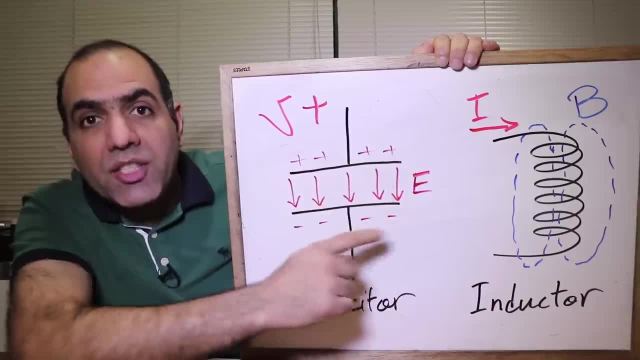 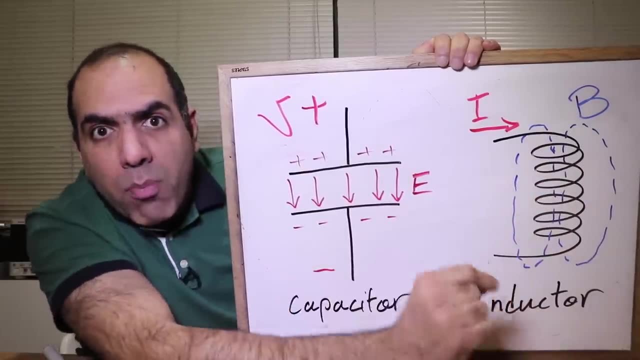 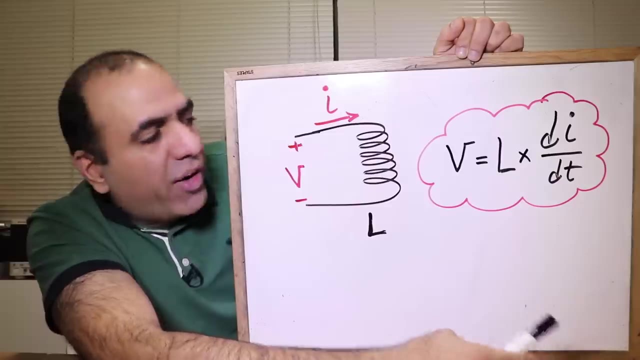 I told you that capacitors store energy in form of electric fields and oppose the change of voltage. Now, inductors store energy as magnetic fields and oppose the change of current. Don't forget that. And here's what we end up calculating through complex math for a relation between voltage and 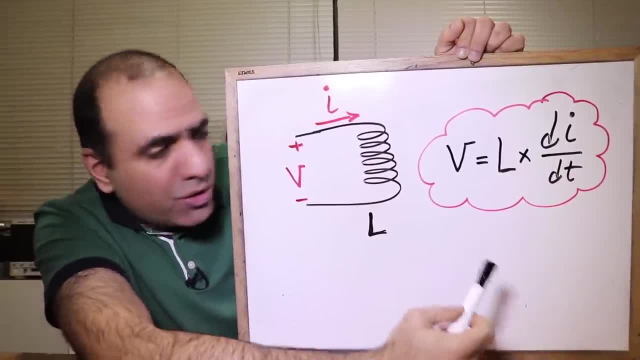 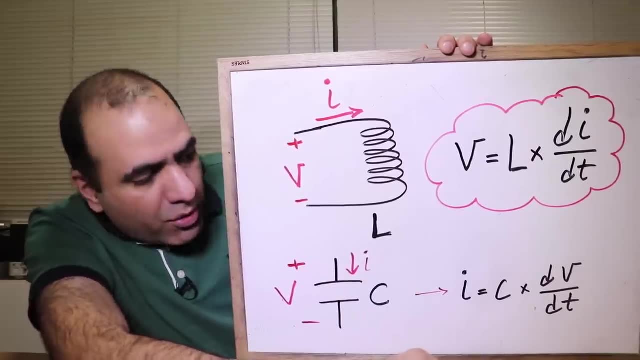 current of an inductor. Basically, the voltage across an inductor is equal to its inductance times, the rate of current change in time, If you remember from the capacitor episode. the voltage across a capacitor cannot change instantaneously in no time, because that would mean 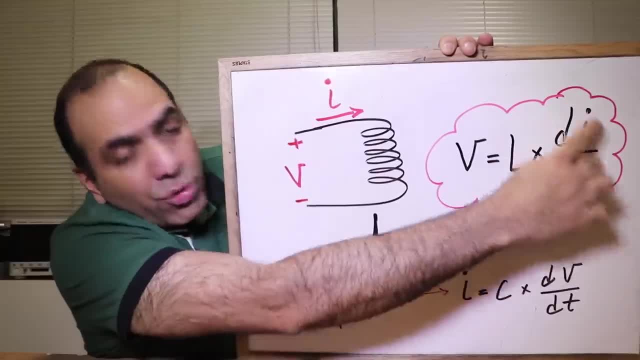 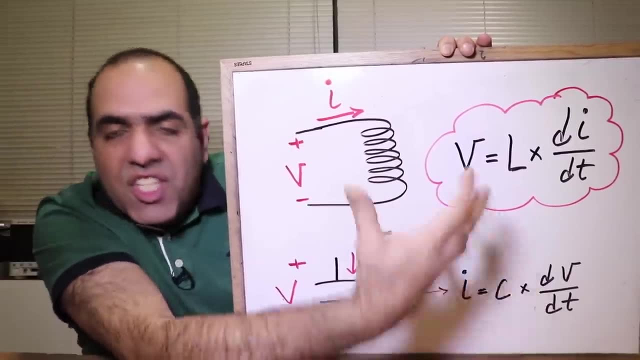 infinite current through the capacitor. Now the current through an inductor cannot change instantaneously because that would mean infinite voltage across it And we can't have this in real life. And that explains what happened at the beginning, when I turned on LEDs by a one and a. 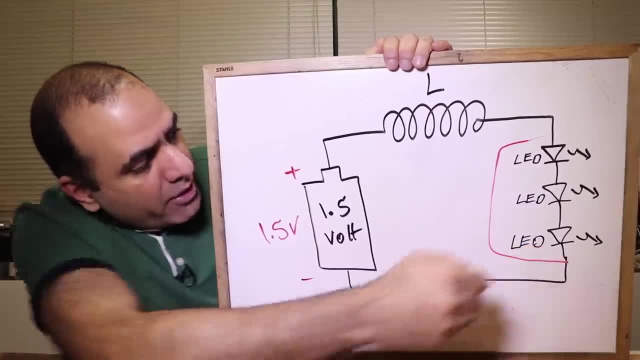 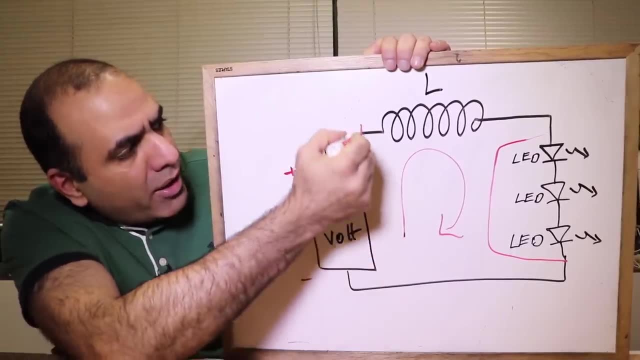 half volt battery. When I short it across the LEDs, I put a DC voltage across the inductor so the current through it williya power over the capacitors gallery box and the voltage across the started to rise, only limited by the resistance of the inductor and the 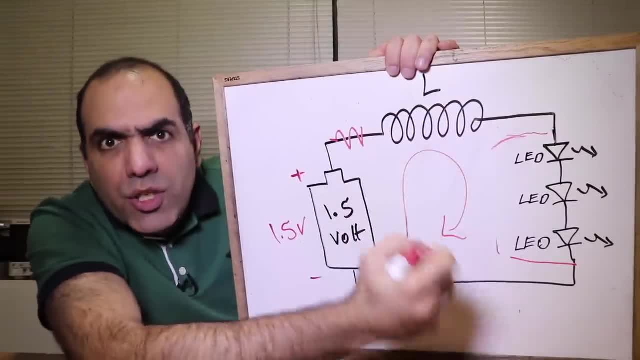 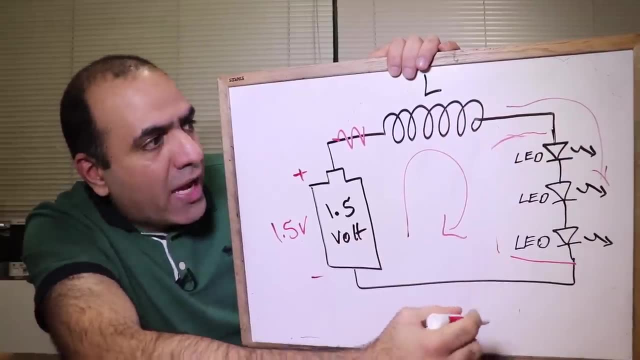 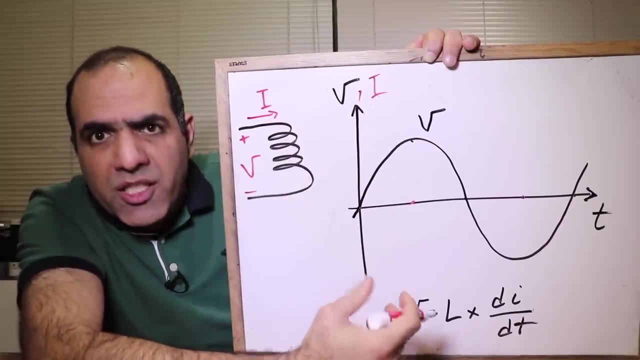 battery. When I opened the short, though, the current through the inductor couldn't change instantaneously as the magnetic fields were collapsing, so it pushed current into the LEDs and the voltage across them instantaneously jumped to 9 volts Also, for example, if the voltage across the inductor changes. 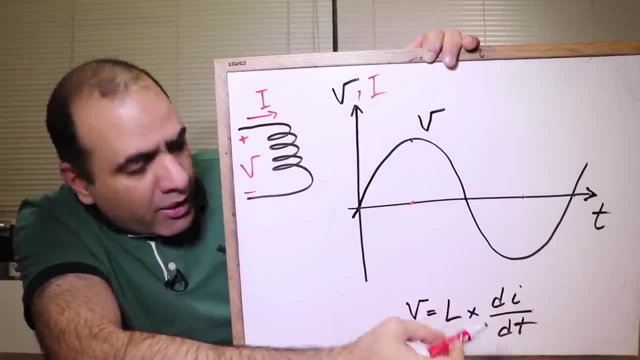 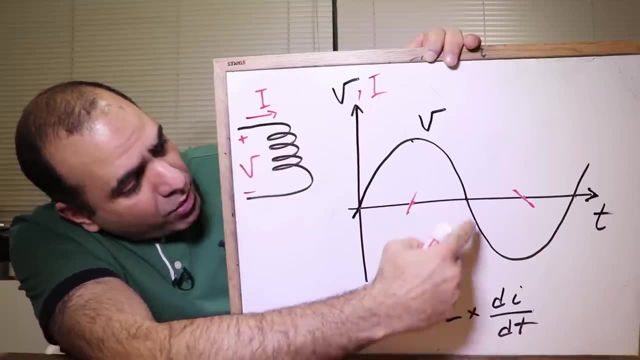 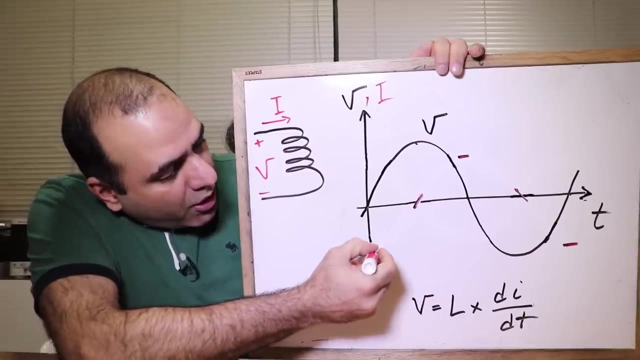 as a sine wave. then when the voltage is at the peaks, it means that the rate of current change is maximum- A positive rate here and a negative rate here- And when the voltage is at zero, it means that the rate of current change is zero here and here. So the inductor current wave looks like this, always lagging. 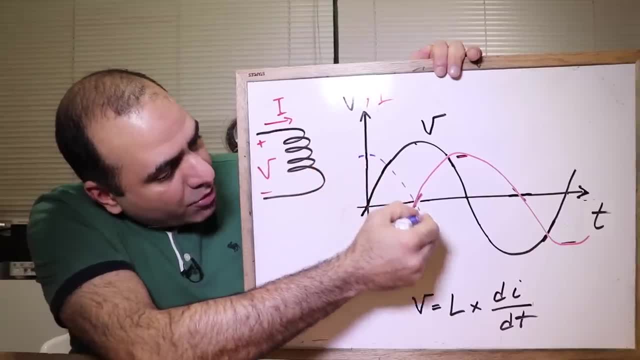 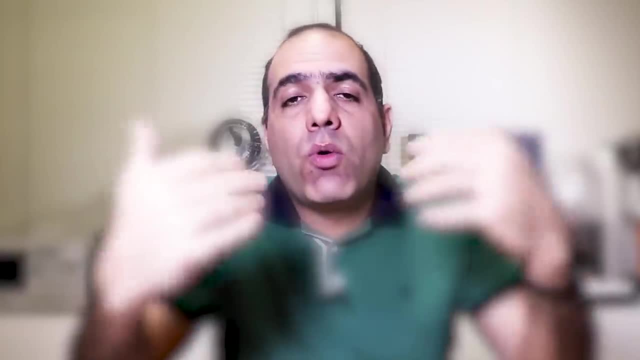 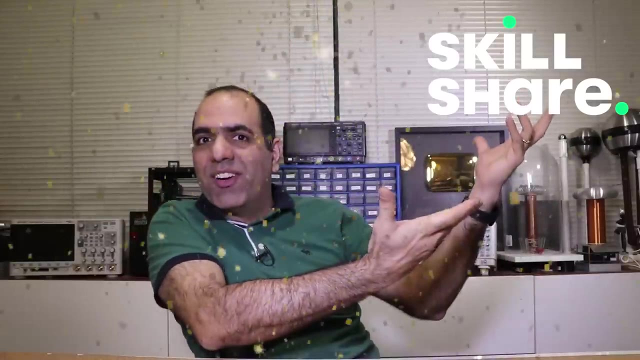 behind the voltage by 90 degrees, unlike a capacitor current that always leads the voltage by 90 degrees. And there we have it. Enough details for one episode. Inductors are beautiful Components like Skillshare, the sponsor of this video. Skillshare is a great. 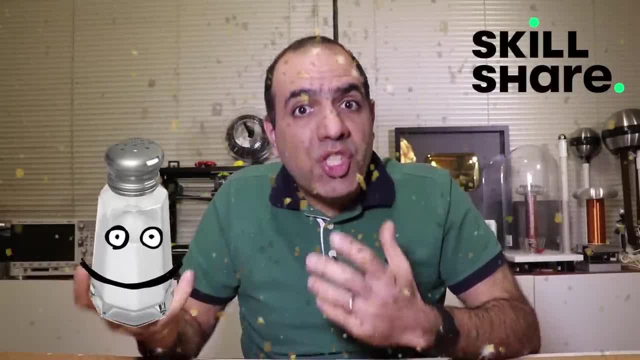 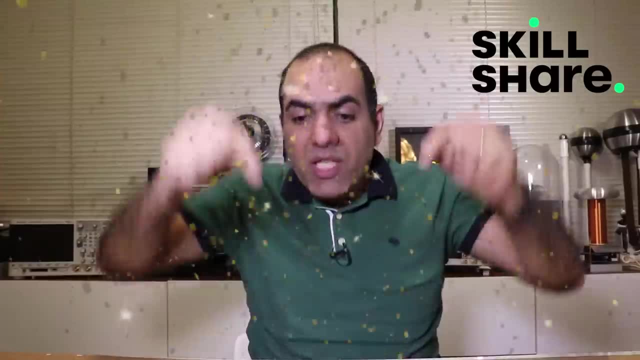 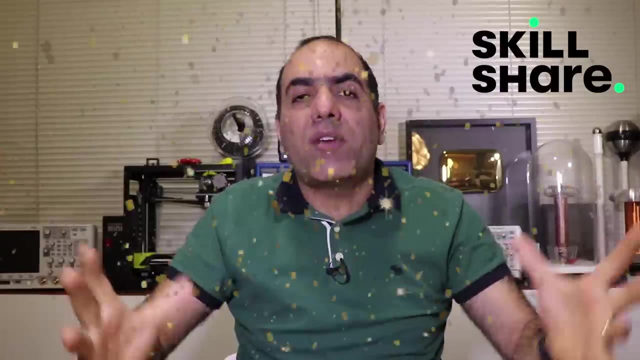 online learning community where people with great skills share them with curious and creative people who want to learn something new or brush up on their knowledge. But wait, Using my link in the description, the first 500 people get two months free trial of Skillshare premium, which is more than enough to take many. 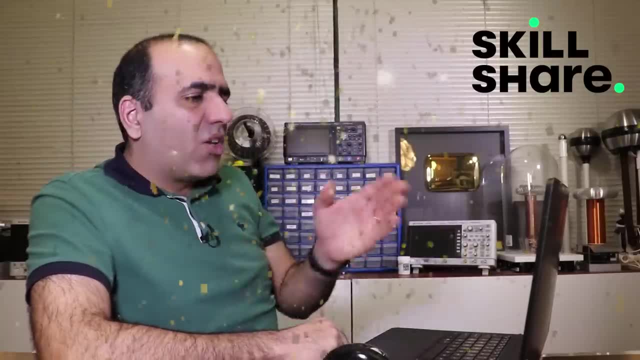 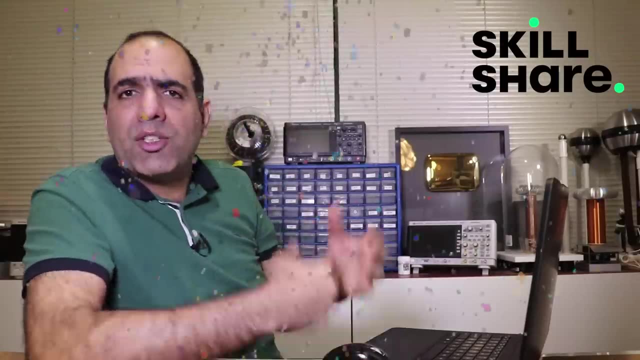 classes and get your feet wet. There are tons of classes on arts, crafts, productivity, film, etc. Film and video production, music, photography and much more. You can take them at your own convenience for as low as $10 a month on a one-year.